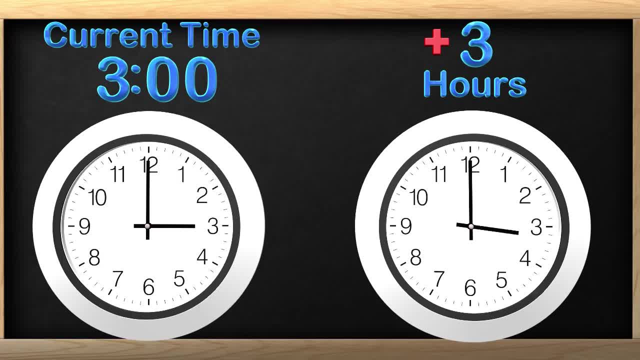 the hour hand and minute hand at the same time. If you know the time of the clock, please hour hand three hours ahead. So we move the hour hand one, two, three hours. It is now pointing at six o'clock, So three hours past three o'clock is six o'clock. Great job, guys. 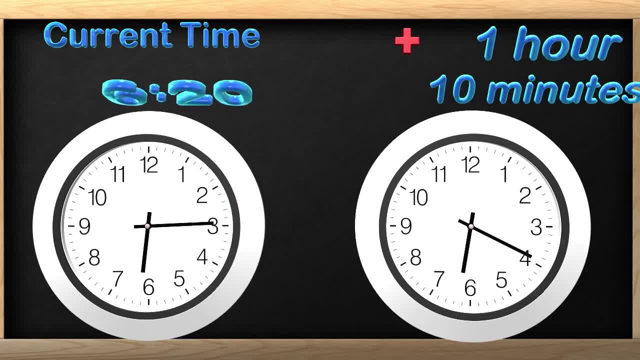 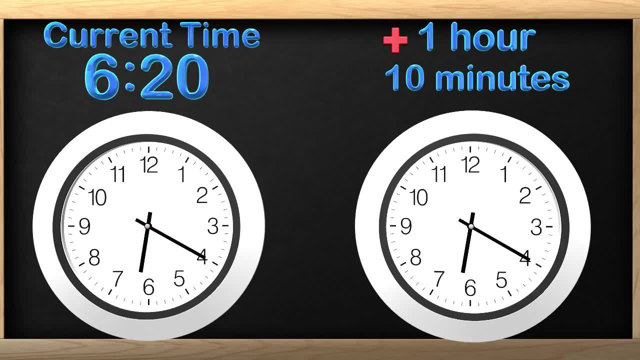 Let's look at some more. Right now the time is 6.20 and my mom said school starts in one hour and ten minutes. What time will it be in one hour and ten minutes? Whenever I get a question like this, I like to imagine how the hands on the clock move, For example: 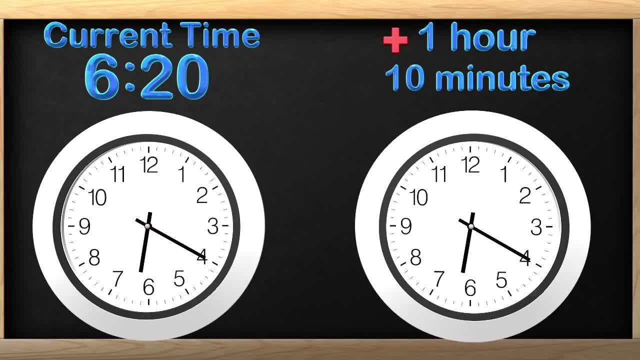 we know that every time the minute hand makes a complete rotation, the hour hand has moved by exactly one hour. Let me show you what I mean. I will move the minute hand all the way around the clock once to show one hour has passed. Did you notice that the hour hand? 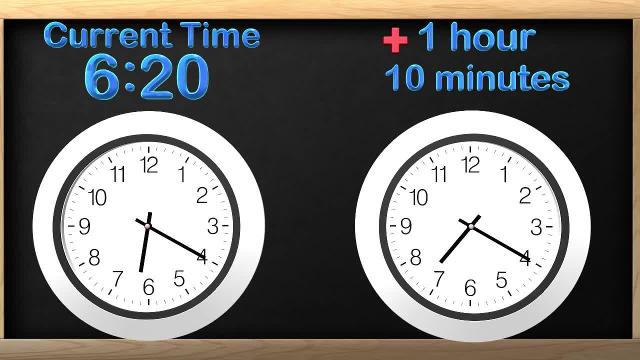 moved as well. We started at 6.20 and we need to know how to know what time it will be in one hour and ten minutes. We just moved the clock ahead one hour. The clock now reads 7.20.. We have moved the time up one hour from 6.20.. Great. 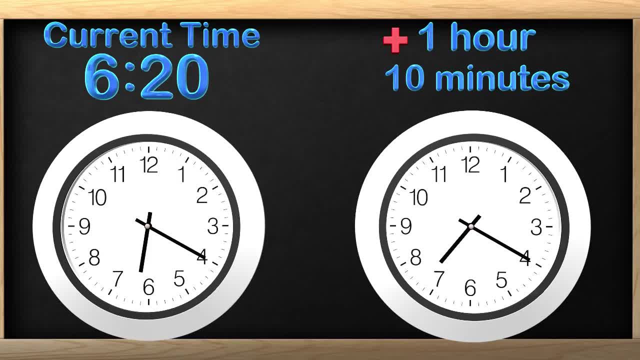 job guys. You are doing awesome. Now we need to move the minute hand forward ten minutes. What is the time now? The time is 7.30.. That is so awesome. So when my mom said school starts at 7.30,, we can see that school starts at 7.30.. Great job, guys. 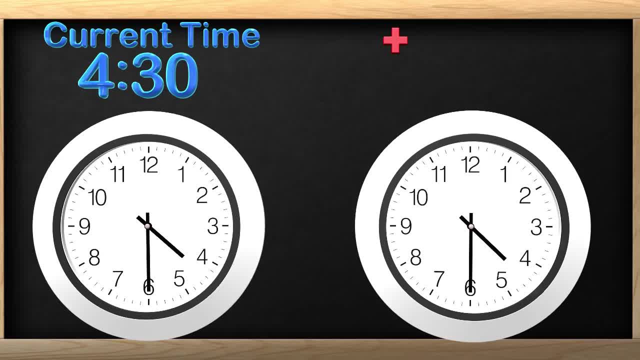 We have seen two problems that we were able to solve, but now I need help knowing when my dodgeball competition is Right. now it is 4.30 and my competition schedule says I need to be at the dodgeball court in two hours and forty-five minutes. I love dodgeball and 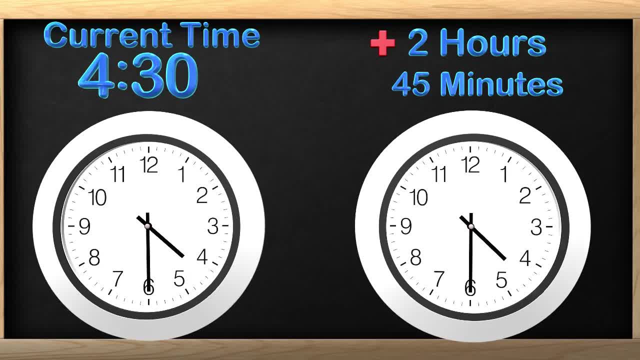 do not want to miss my competition, so let's figure this out. Since we have another clock here to use, let's move the hands ahead, starting with the minutes. Now. we need to remember that when the minute hand moves all the way up to the 12, it starts a new hour. That means